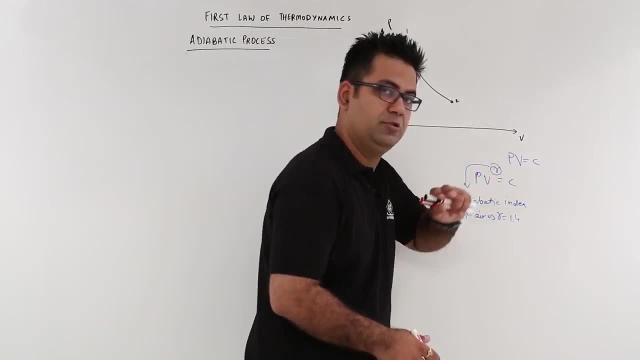 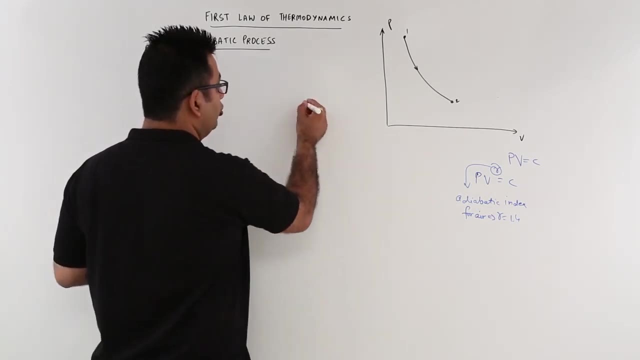 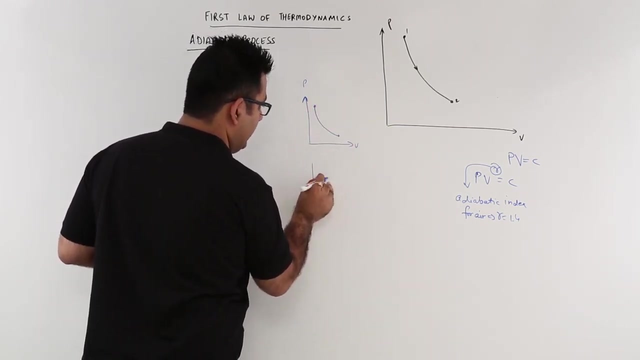 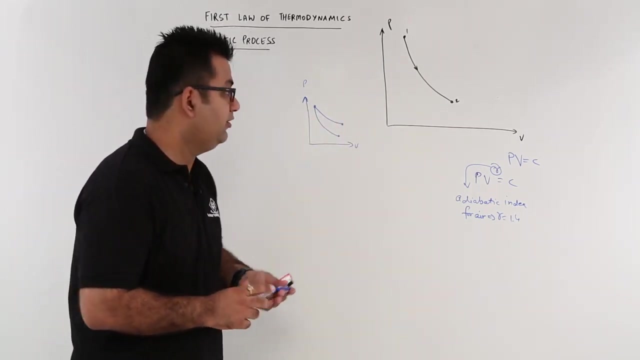 equation for adiabatic process and this is for isothermal. This means that the difference Now, how do you differentiate? Because if you look at the two graphs, this is PV and let me draw it on the same plot, this, Between these two graphs, which one is showing the isothermal and which one is? 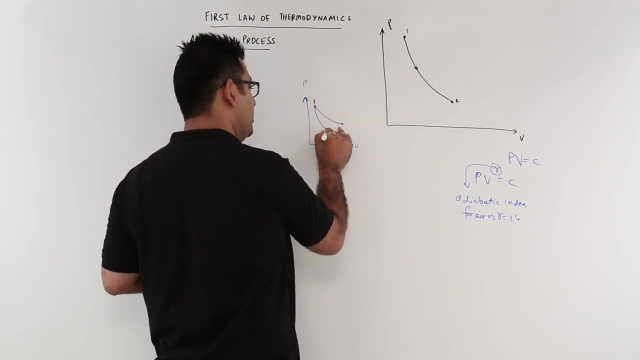 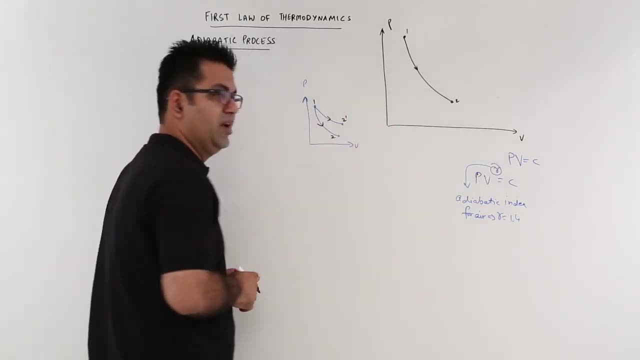 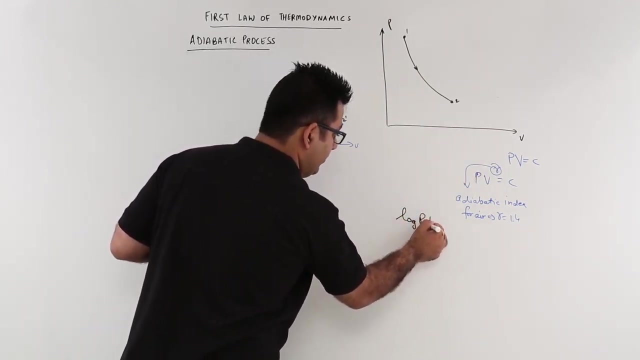 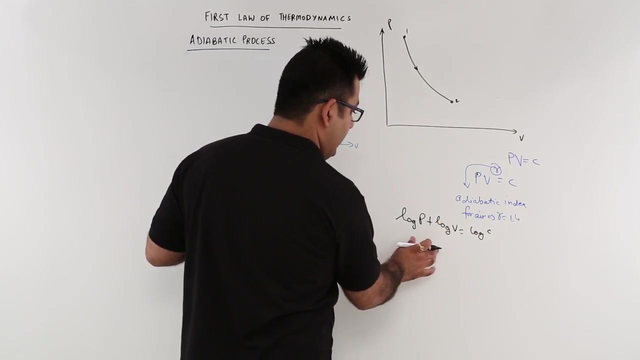 showing the adiabatic. Let's have 1. 2,2 dash. Now, if you look at these two equations and you take log on both the sides, you will get log P plus log V is equal to log C. Ok, Now take V on that side, So you will have. 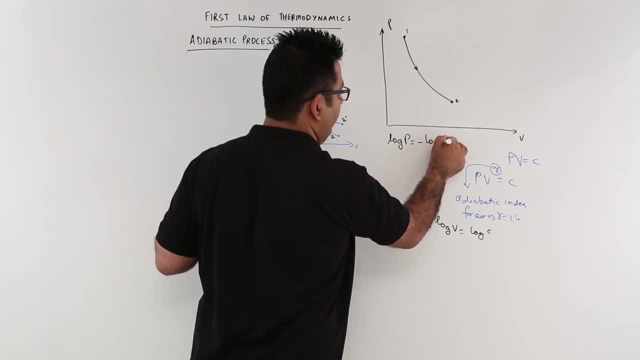 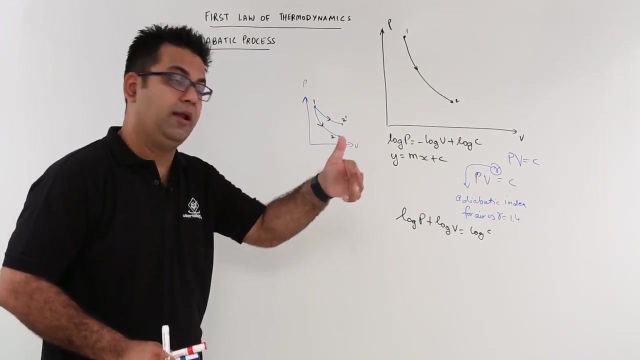 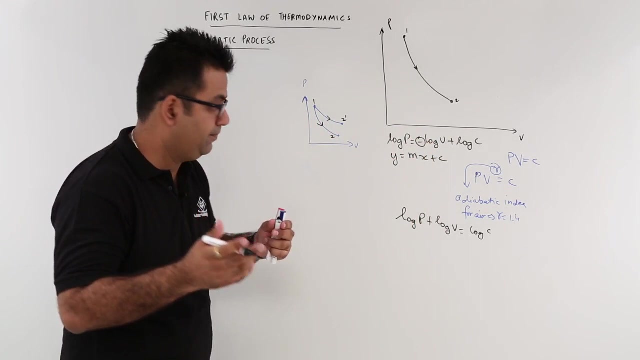 log P is equal to minus log V, plus log C. Ok, So let me just put this analogous to the straight line equation. So if I convert this curve to a straight line, you get this kind of an equation, okay, where this part is the slope minus 1, okay. 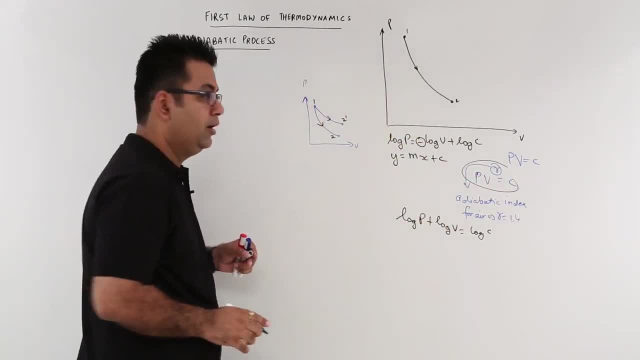 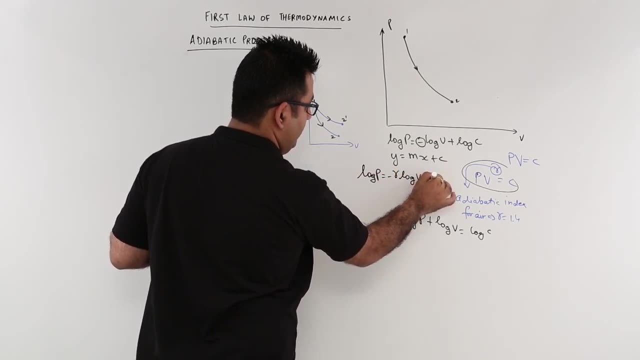 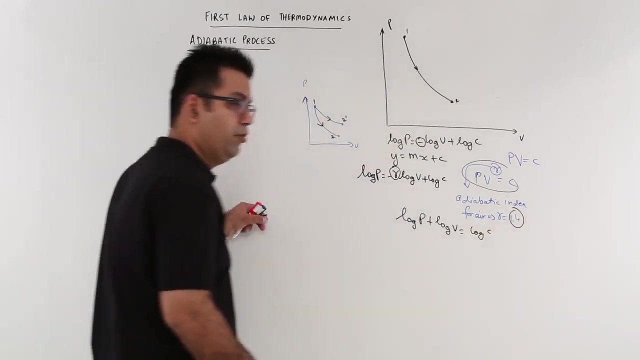 If you convert this into a straight line, you get: log P is equal to minus gamma, log V plus log C. Now in this case the slope is gamma Gamma, let us say, for air is 1.4.. In both the cases we are using air. 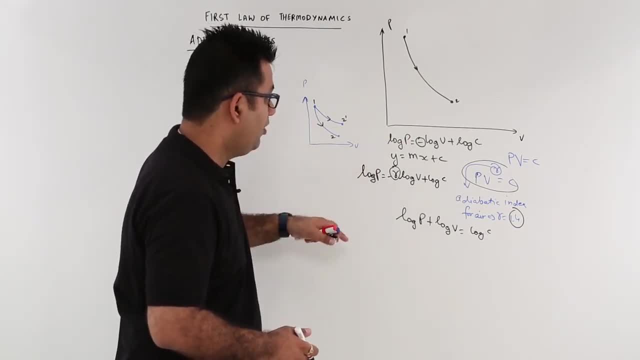 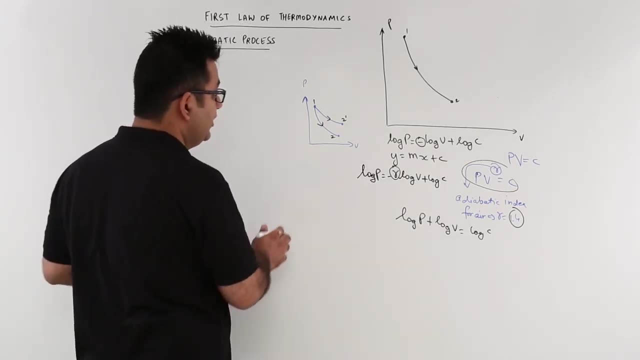 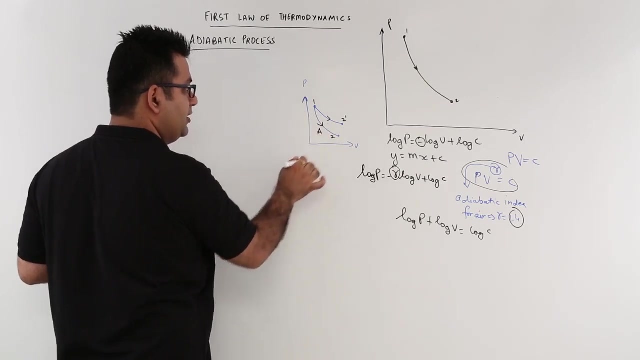 So for air, the slope of an isothermal curve is less as compared to the slope for an idiomatic process. This means This means the curve which is, you know, which has a higher slope, will indicate an idiomatic process and the lesser slope will indicate an isothermal process. 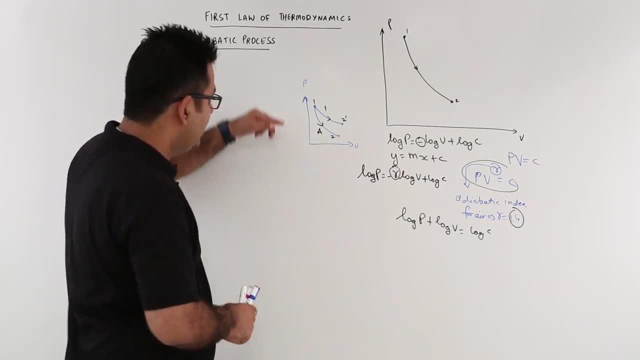 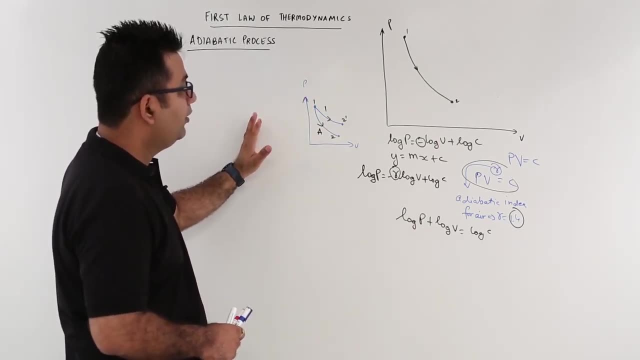 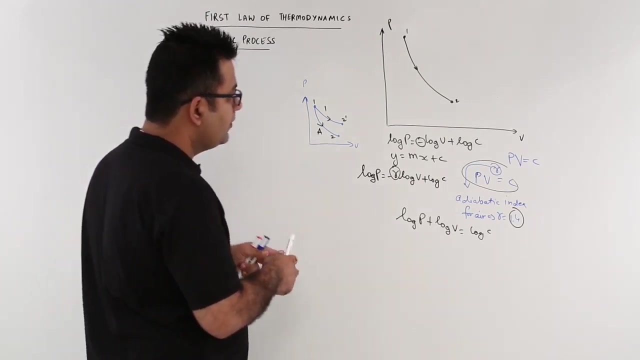 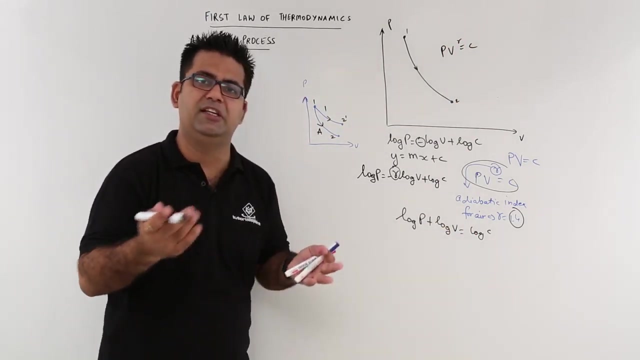 So the differentiating vector is the steepness in the slope or the steepness in the curve of these two processes. So this is how you differentiate between an idiomatic and an isothermal process curve. right Now, the The mathematical equation is: PV to the power. gamma is equal to constant. Now, what is constant in this? 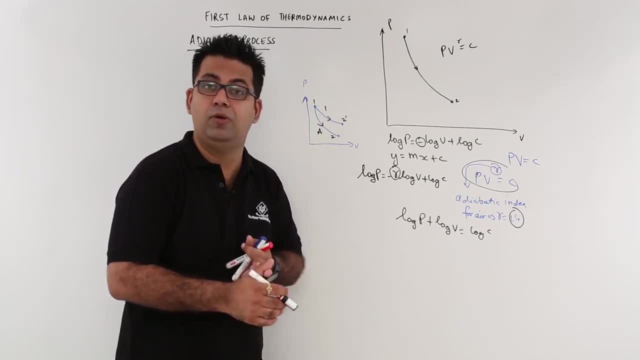 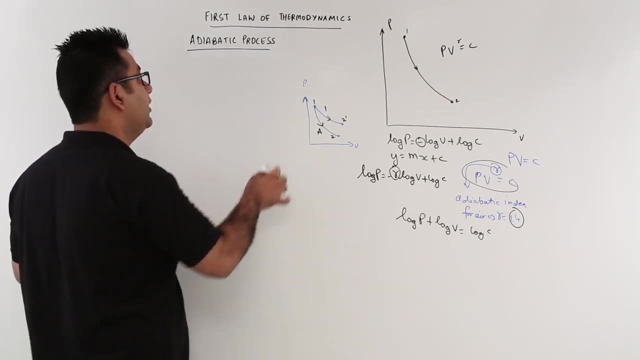 In isobaric you had pressure constant. In isochoric you had volume constant. In isothermal you had temperature constant. Now, what is constant in idiomatic? In idiomatic there is no heat flow. Q is equal to 0.. 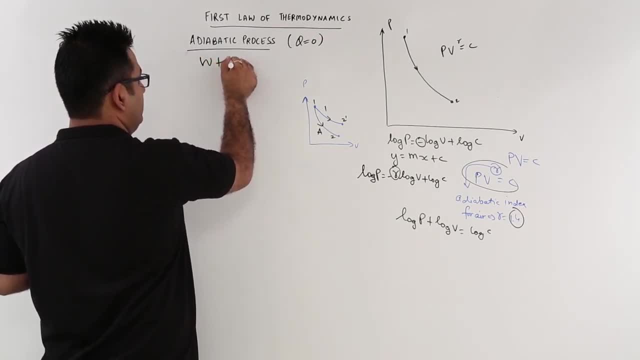 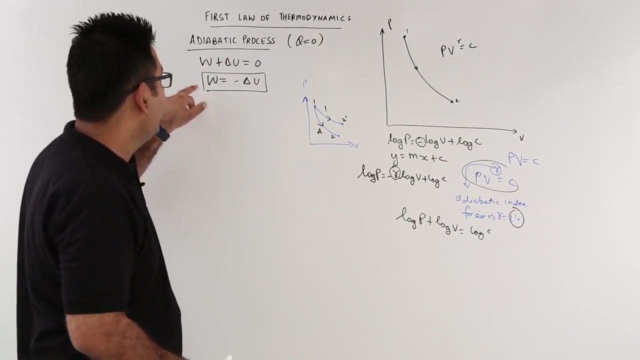 So if you apply the first law, this is what you get. okay, And this will give you. W is equal to minus delta U. This means whatever work that you get as an output, it is at the expense of the internal energy. 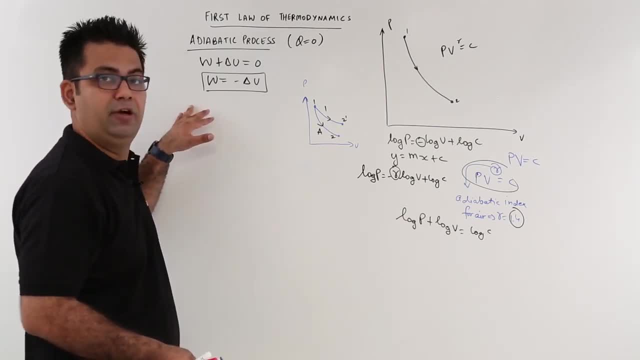 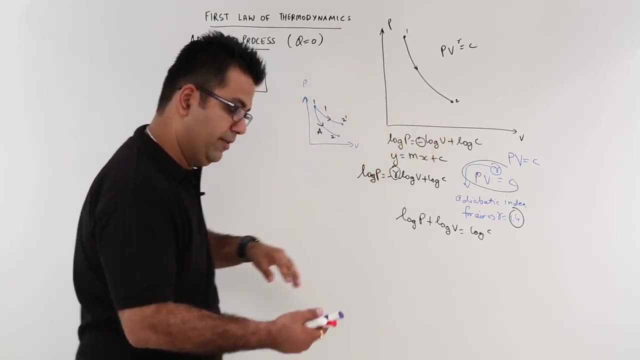 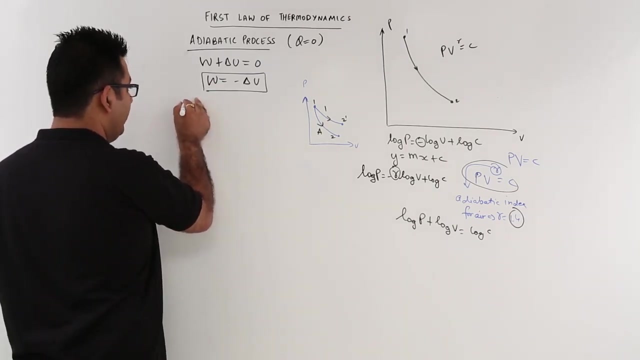 So a decrease in the internal energy converts itself into the work output. okay, So this is the you can say analysis of an idiomatic process. Now, if you find out the work done, that is W. So we know that W1, 2 is equal to integral, V1 to V2, PdV. 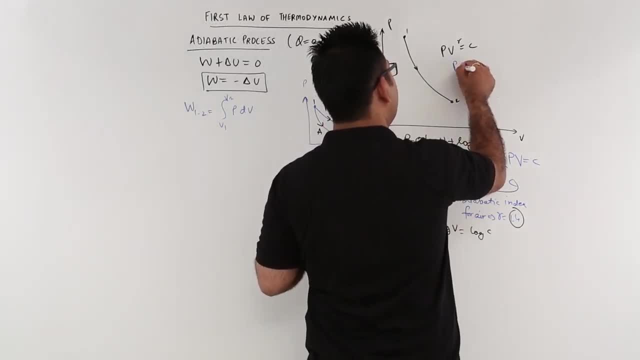 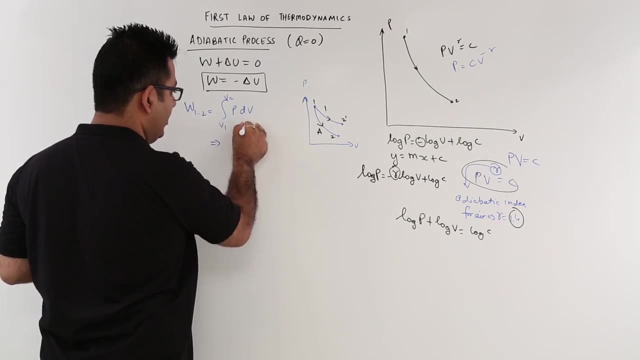 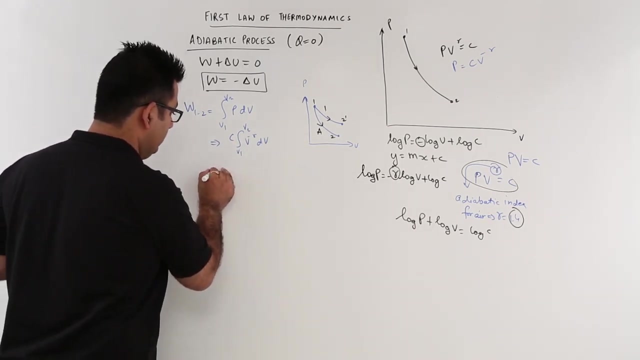 And I know the value of P from here. So the value of P would be C into V to the power, minus gamma. So this would be equal to integral V1 to V2, C constant minus gamma, dV. okay, So this would come equal to C into V to the power. 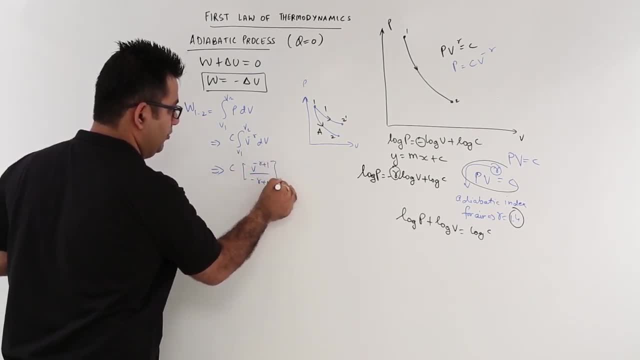 Minus gamma, plus 1 upon minus gamma, plus 1 upon V1, V2.. So when you resolve this, you get C into into. you get V2, 1 minus gamma minus V1, 1 minus gamma upon 1 minus gamma. 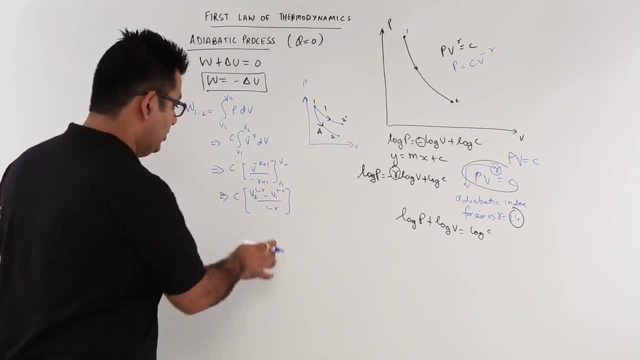 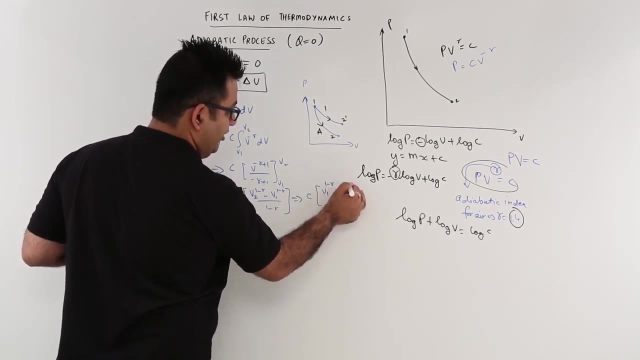 Now, gamma is higher as compared to 1. So this would be a negative value. You can take a negative as a common value, So you get 1 minus gamma, V2, 1 minus gamma And this becomes gamma minus 1.. 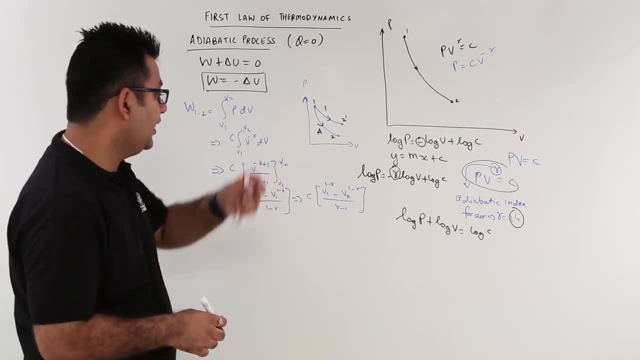 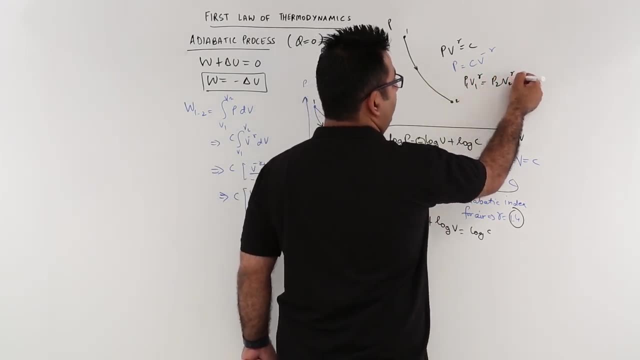 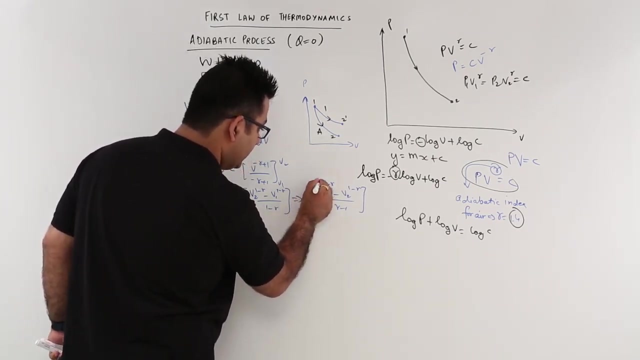 Alright. Now, if you look at that equation, you get P1. V1 to the power gamma is equal to P2. V2 to the power gamma is equal to C, Isn't it So, the value of C. if you multiply this C with this, I can substitute for P1: V1 to the power gamma. 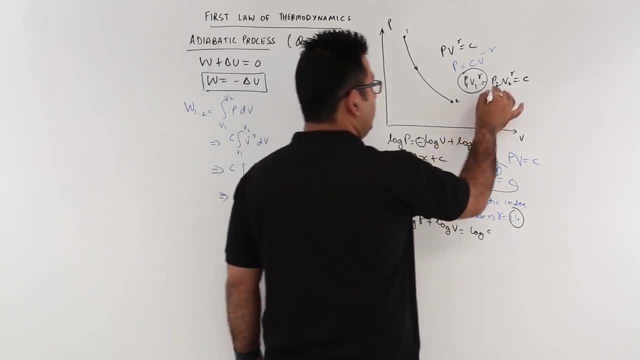 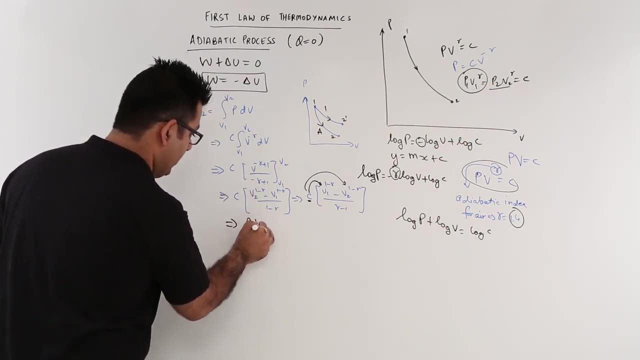 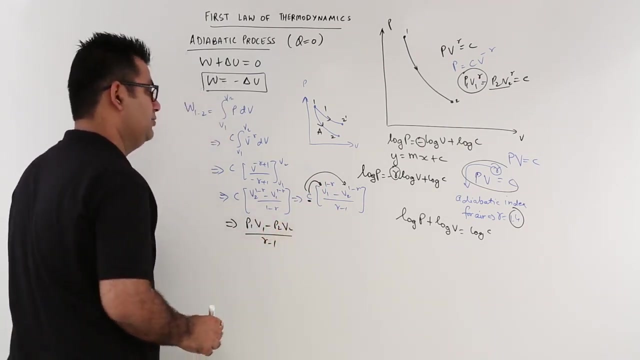 If I multiply this C in this term I can substitute. I can substitute for P2, V2 to the power gamma, So this would come P1 into V1, gamma would be cancelled in the power minus P2. V2 upon gamma minus 1.. 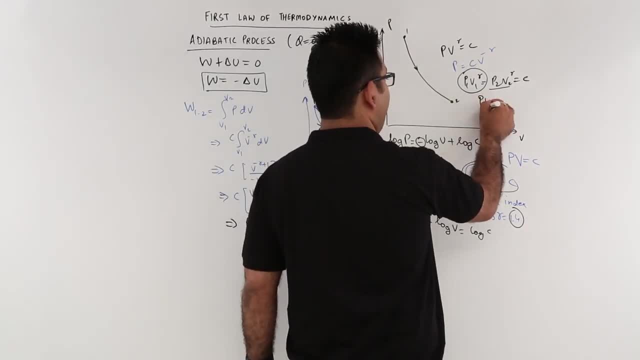 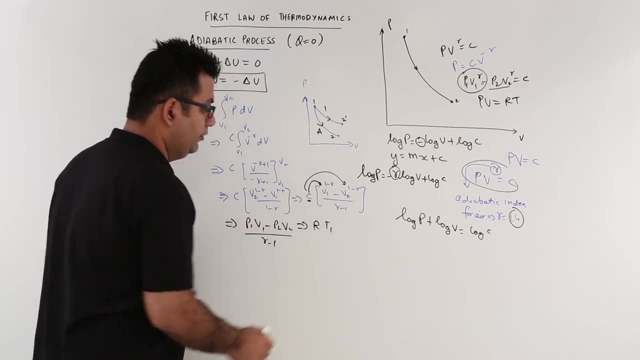 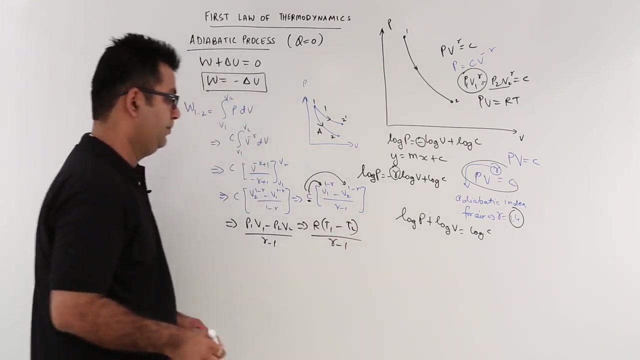 Okay, Now this PV, this is equal to what RT. So you can substitute P1- V1 as R into T1 and P2- V2 as R into T2.. So R. So R becomes constant, and this is gamma minus 1.. 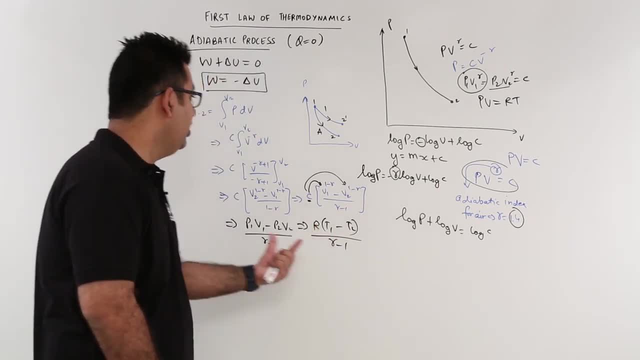 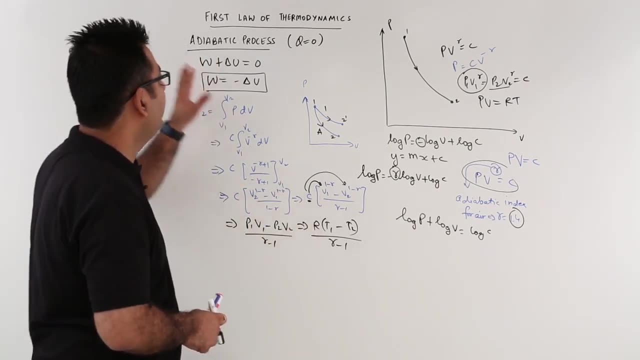 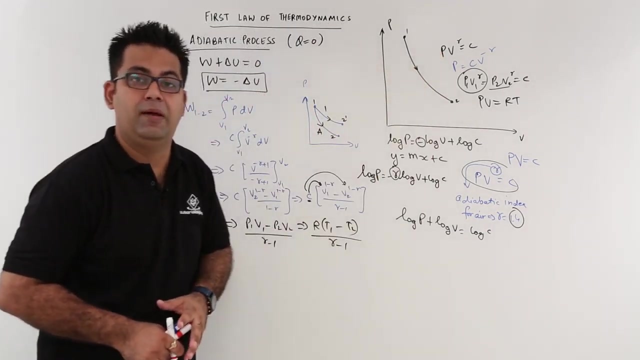 So this mathematical expression is the value for work done in an adiabatic process. Okay, So I hope you understood this analysis on adiabatic process which has Q equal to 0 and the mathematical equation governing it is PV to the power. gamma is equal to constant. 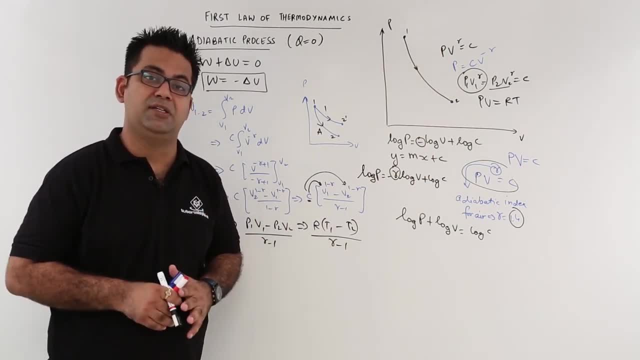 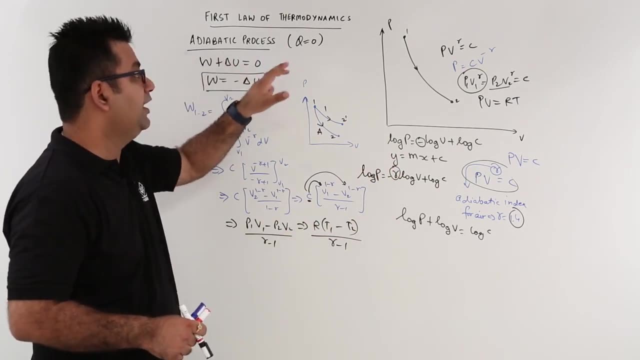 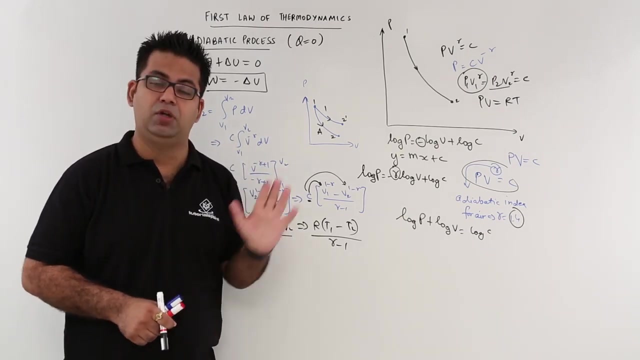 Now we are done with the four non-flow applications of the first law. Now, all these Are only possible if the processes indicated in this are quasi-static in nature. Okay, So now, after this, let us look at some examples on these four non-flow processes.